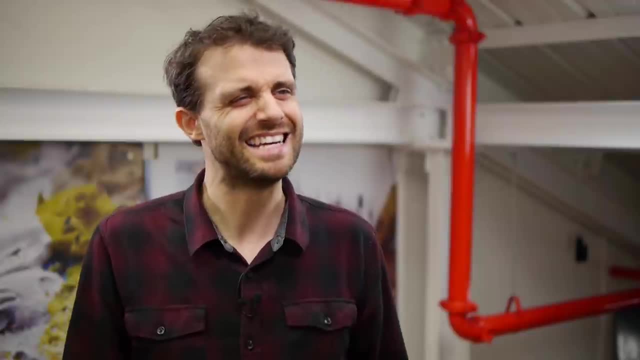 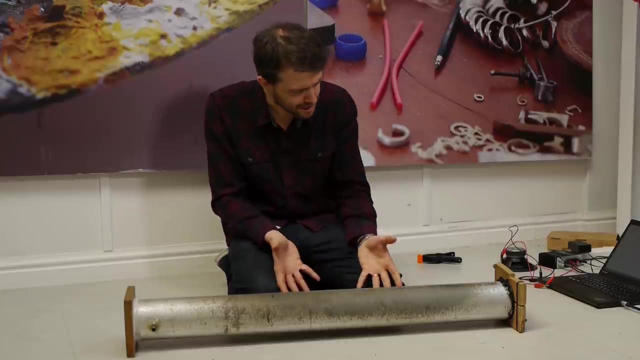 resonant frequency of that object, and that's resonance. It's okay as a description, but I think I can do better. The best way I've found to describe resonance is using this thing. It's called a Rubens tube. It's a hollow aluminium tube. At one end it's blocked off with a piece. 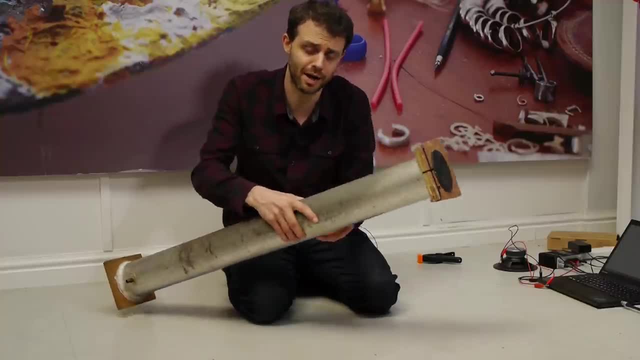 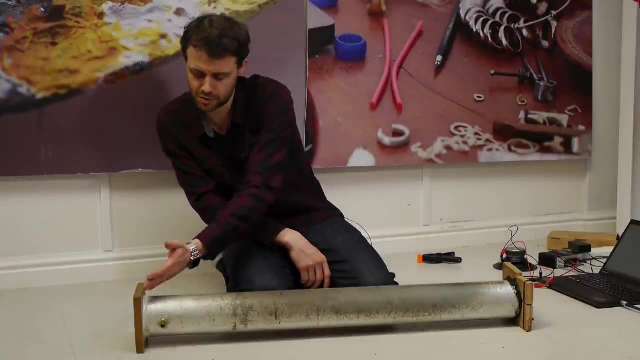 of wood. At the other end it's blocked off with a piece of wood. At the other end it's blocked off with a rubber membrane and if I tap that membrane with my finger then that will send a pulse of pressure through the tube, traveling at the speed of sand. When the pulse reaches this end, some of 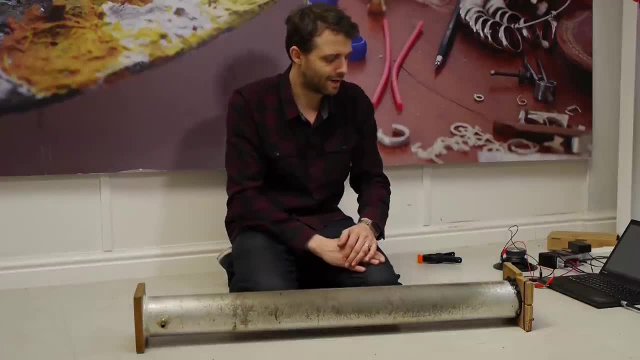 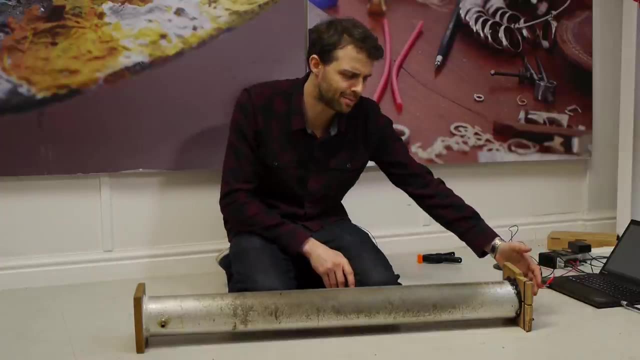 it gets reflected and it travels back through the tube to here, and then, when the pulse gets to here, some of it gets reflected and it travels back in this direction. So when I tap the rubber membrane, a pulse of pressure bounces backwards and forwards and it's reflected back in this. 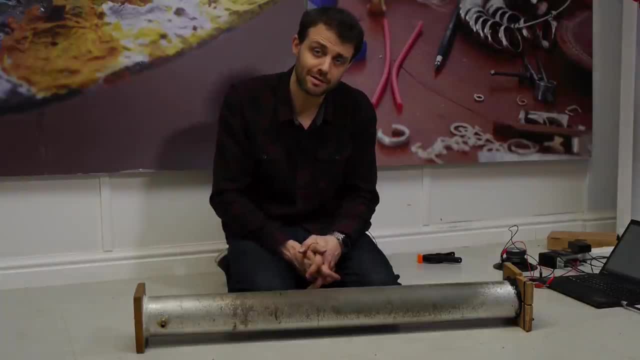 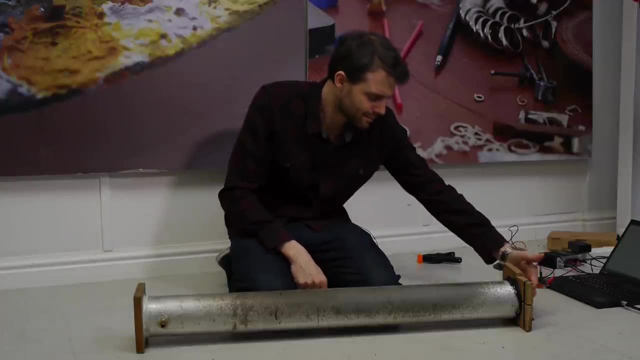 direction. So when I tap the rubber membrane, a pulse of pressure bounces backwards and forwards inside the tube, getting weaker and weaker, and weaker, until eventually it fades away to nothing. But what if I repeatedly tap the rubber membrane? So I tap the rubber, the pulse passes through the. 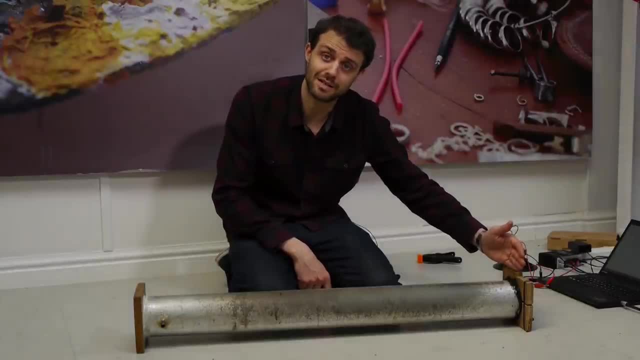 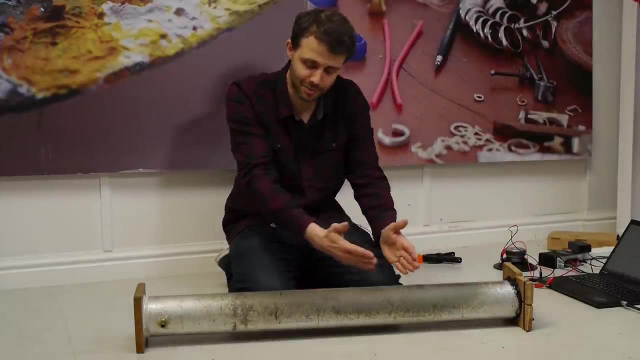 tube. it bounces off here, it comes back to here and just as it reaches this side I tap the membrane again and now the pulse is even bigger than it was before because I've added to it. So now a larger pulse is traveling through the tube. it bounces back, gets to here Just when it gets. 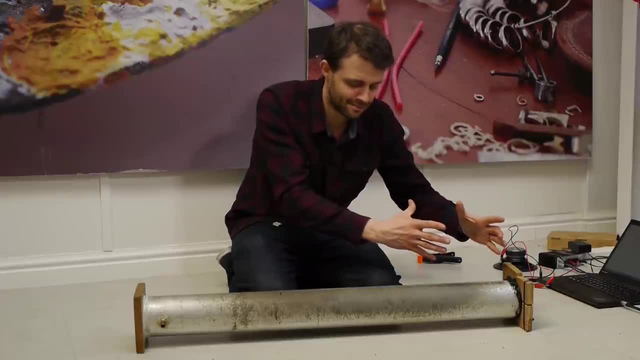 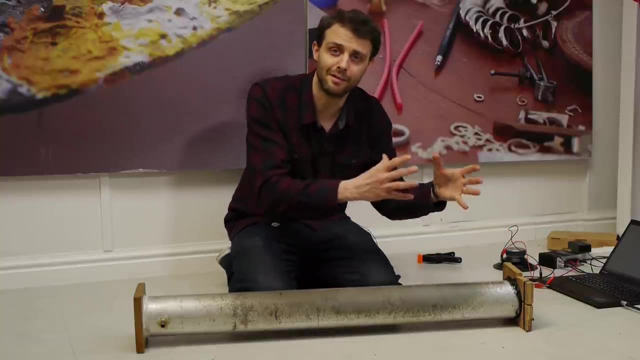 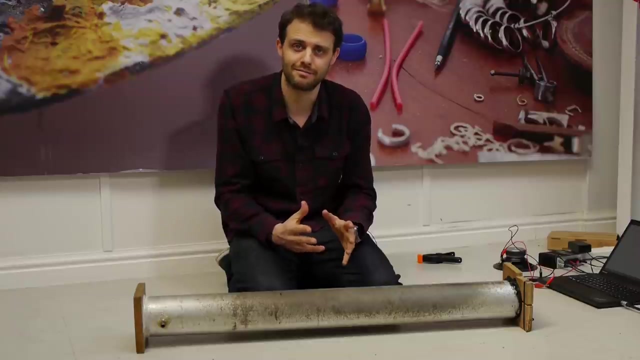 bigger. I tap it a third time and now the pulse is even bigger again. And if I keep doing that, if I keep tapping the rubber membrane at just the right time, the pulse will get bigger, and bigger and bigger. And that's resonance. Resonance is getting the timing just right, getting the 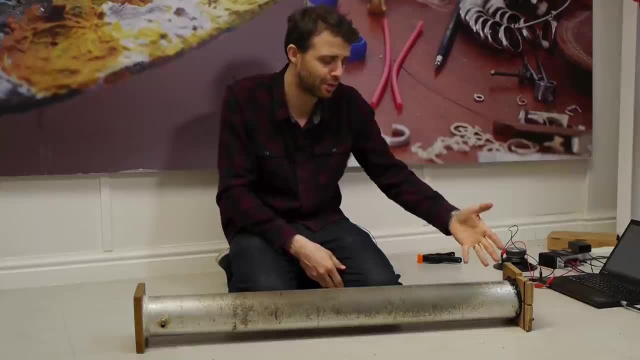 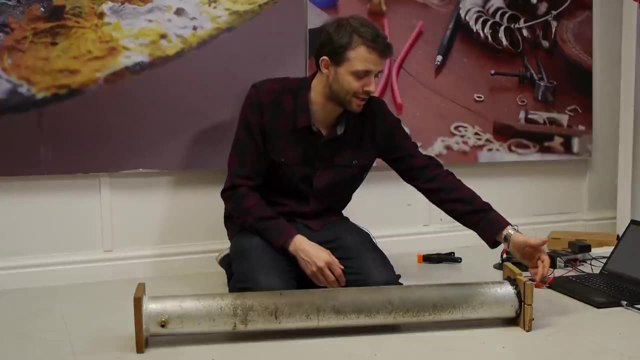 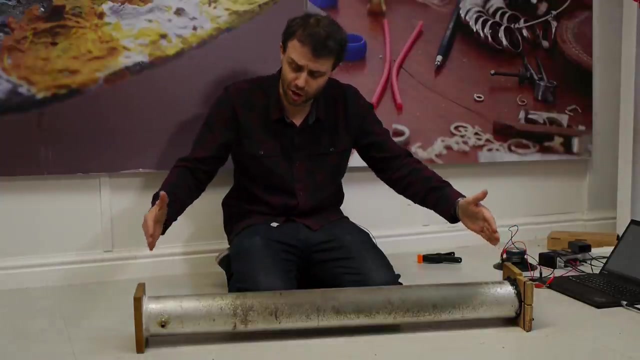 frequency just right, so that the energy you put into the system adds to the energy that's already there. That's resonance. So the frequency of taps that I need to, that I need to get, that's the resonant frequency of the column of air inside. 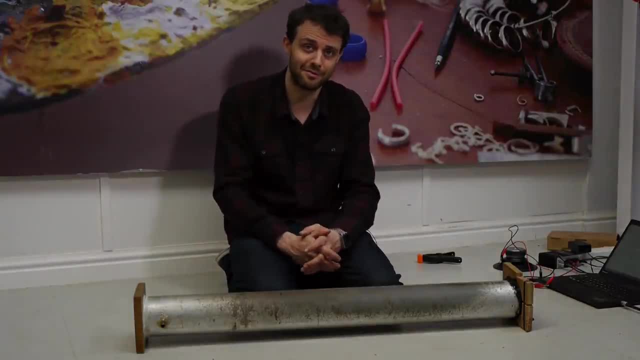 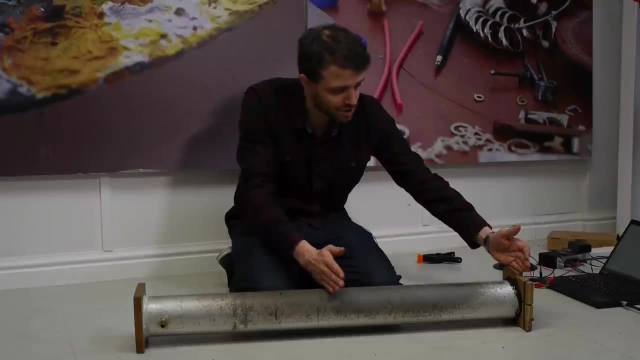 this tube. But it's not the only resonant frequency of the column of air. There are infinitely many. So, for example, if I tap the rubber membrane and a pulse goes into the tube and then I tap it a second time, so now there are two pulses inside the tube. look, they cross over like this: And: 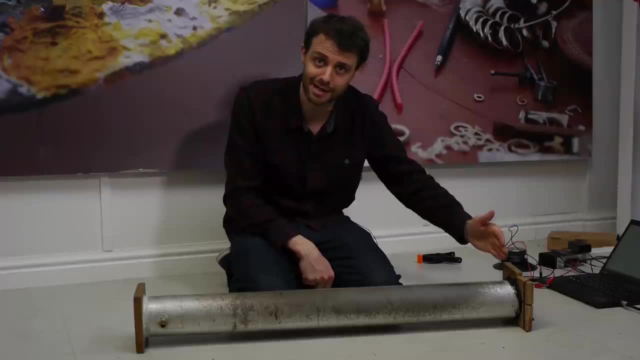 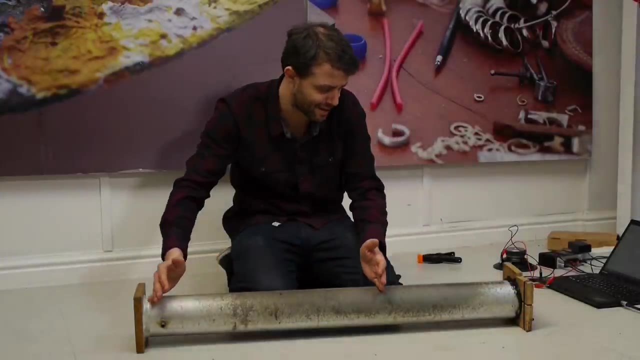 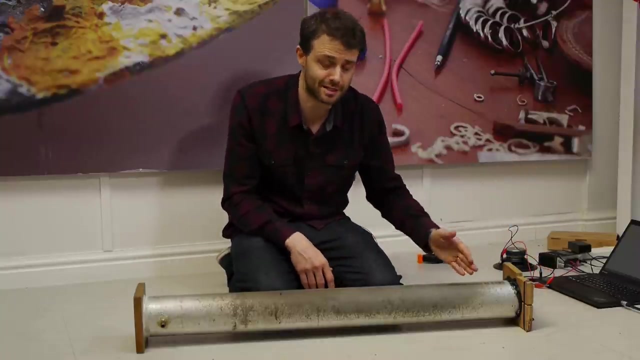 then the third tap happens when the first tap gets back. Or I could tap the rubber membrane twice, so you know, one goes in, another one goes in there maybe, and then a third one goes in, like that, And then the fourth tap doesn't happen until the first one gets back. But I'm 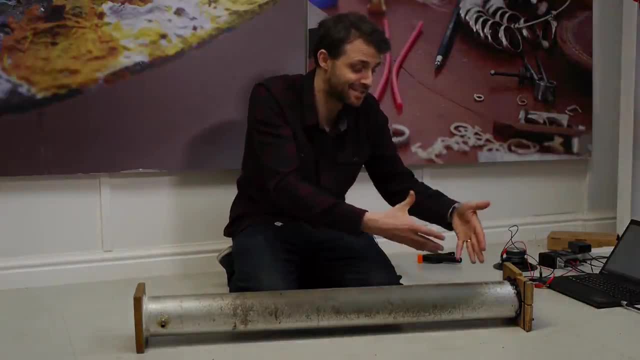 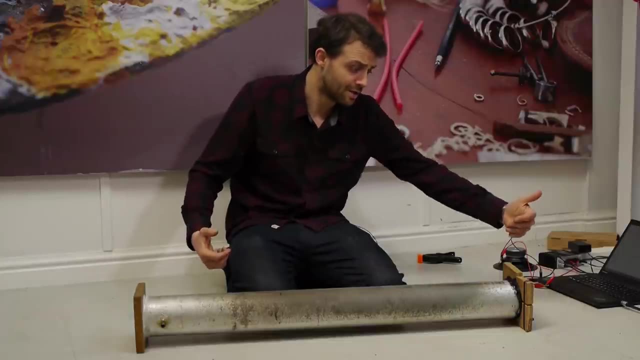 still getting the timing just right, so that the energy I put in adds to the energy that's already there. It's just that I've waited for a couple of taps to go in first. So what's that like when you've got pulses coming in from this direction and the reflected pulses coming back and they're 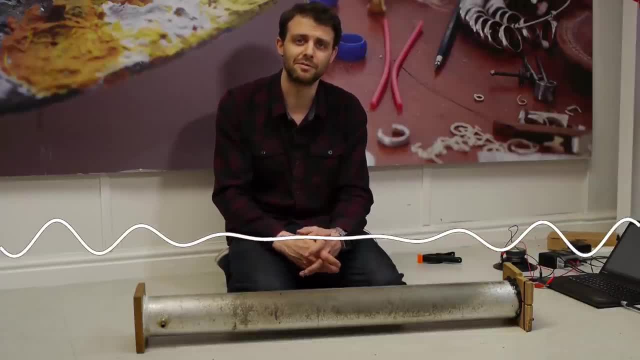 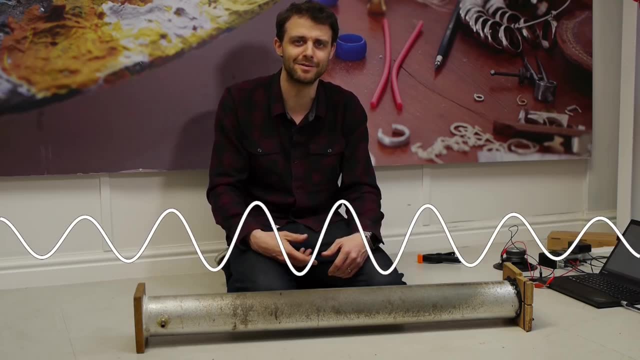 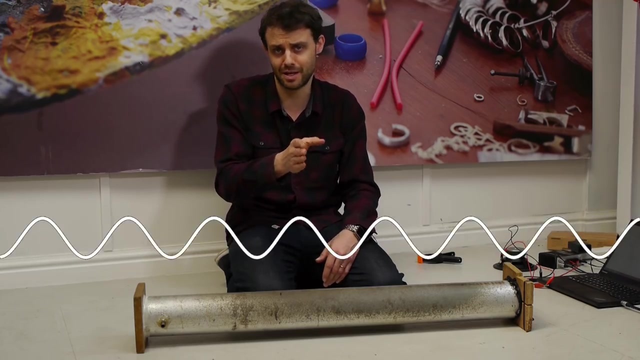 crossing over each other. It looks like this. So the waves coming from both directions, they cross over each other and they add together, And when you add them together you get something called a standing wave, where you have nodes and antinodes. The nodes are the points where there's no movement and the antinodes are the points where 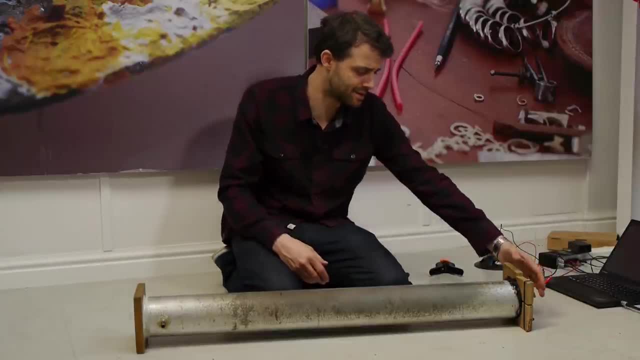 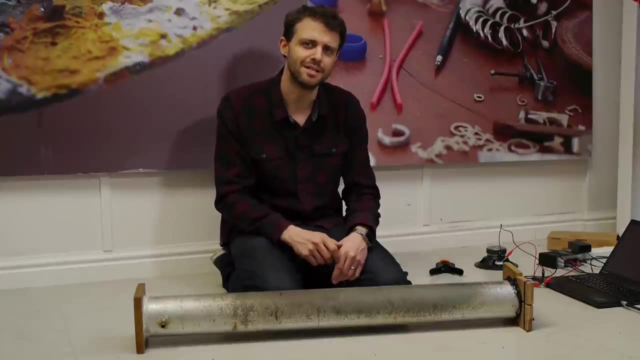 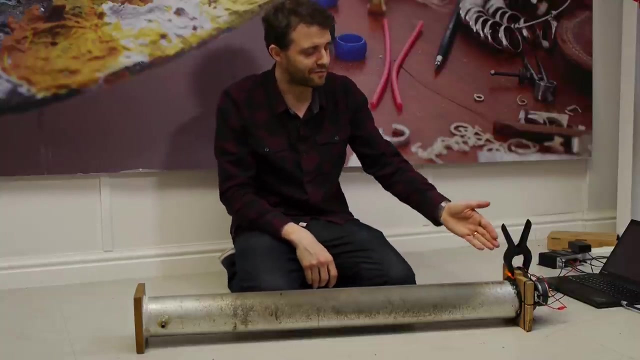 there's lots of movement. So how fast do I need to tap this membrane to see the effect? Well, much faster than I can tap with my finger. In fact, it's an audible frequency. so instead of using my finger, I'll attach it. I'll attach a speaker to the end, like this. So if I can drive the speaker at the resonating 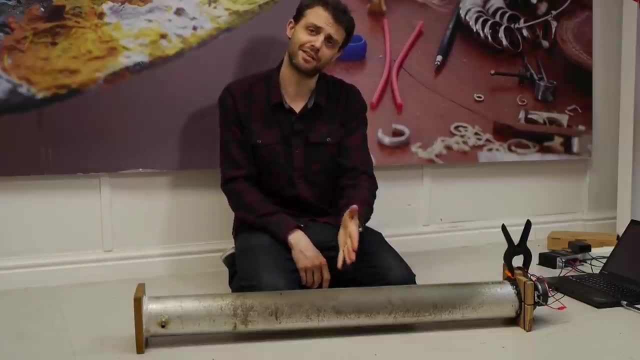 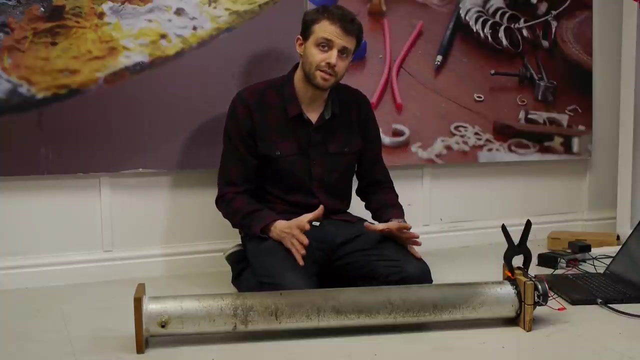 frequency of this tube, then the energy that I put into the system adds to the energy that's already there and we should hear that as an increase in the amplitude of the sound. We should hear the volume go up. So let's try that. Okay, so this isn't one of the resonating frequencies of the 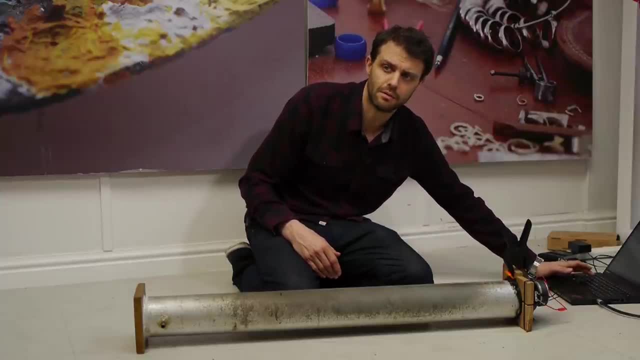 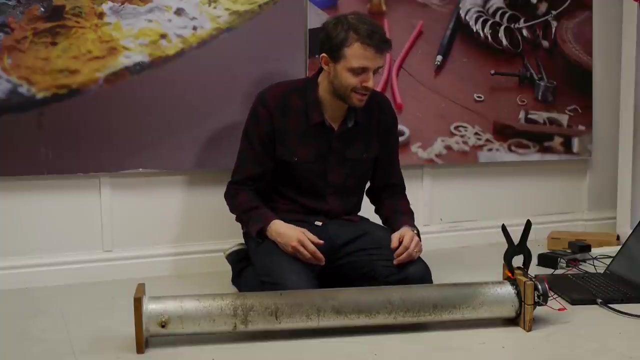 tube. But if I just bump up the frequency a little bit, Okay, so the volume went up. I've found the resonating frequency of this tube. This speaker is tapping the rubber membrane at just the right speed so that the next tap of the speaker is. 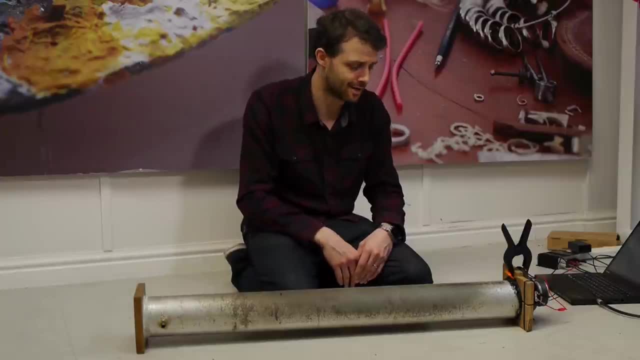 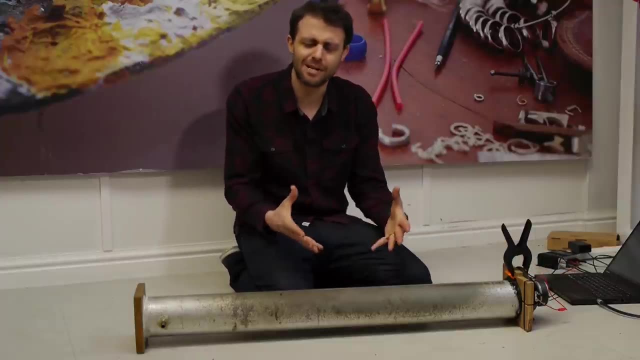 meeting one of the returning pulses from this end and we're adding to the energy that's already in the system. That's resonance. The problem is what's happening? because it's happening inside the tube and air is invisible, which is why the Rubens tube is designed to be set on fire. Before I set anything on fire, I've actually switched out. 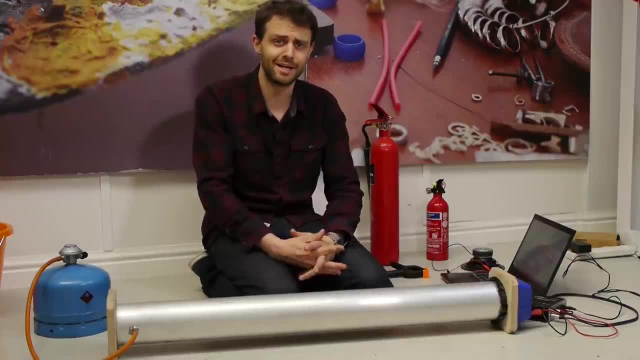 the Rubens tube. The first one I showed you was one I built myself and it was a while ago and I didn't know what I was doing, and it's a little bit worse for wear, so I wasn't comfortable setting that one on fire. This is one that I bought. The only problem with this one: 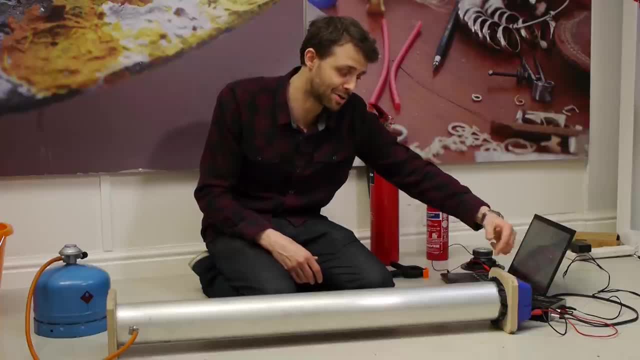 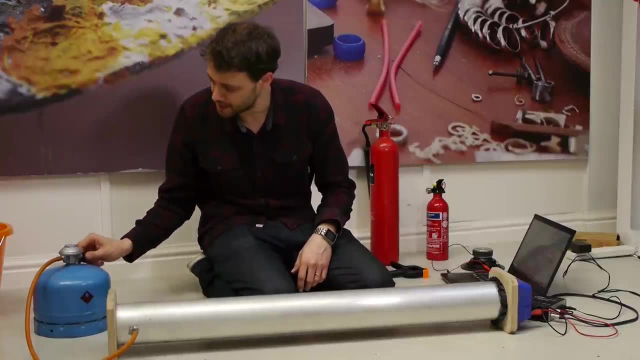 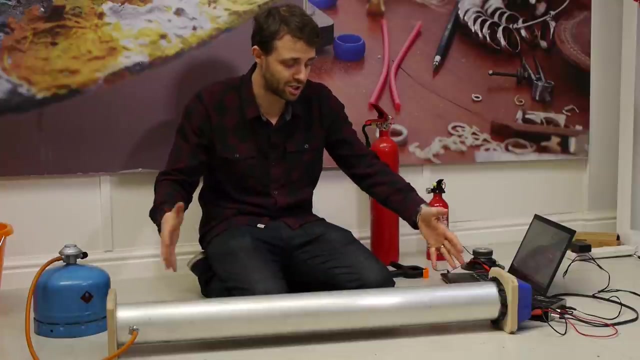 is that the speaker assembly is completely enclosed, and I really wanted to show you the rubber membrane and the whole tapping thing. With this one I'm comfortable to set it on fire, So we pump in butane through here and then we set light to it. The first thing you have to do is fill the 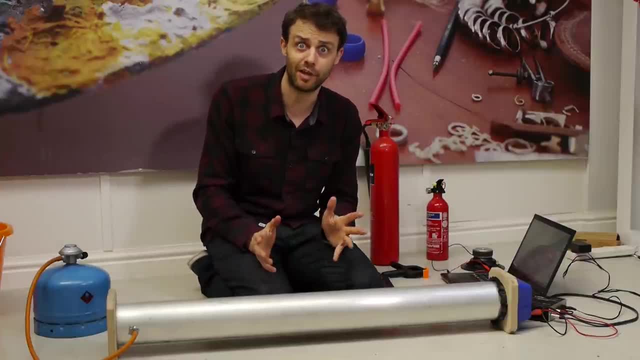 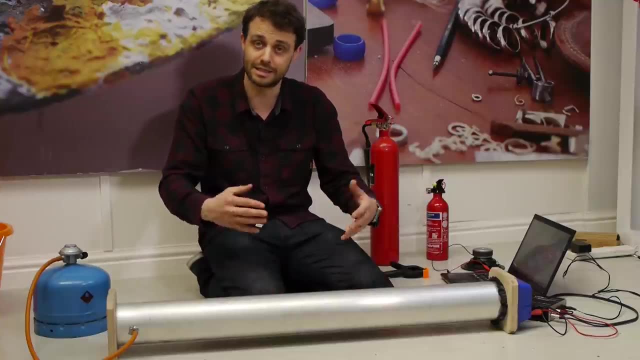 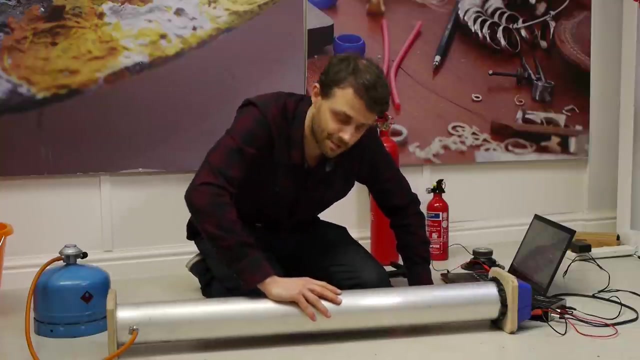 tube with butane. Basically you have to get past 15% butane because that's a dangerous mixture. It's a stoichiometric ratio and it's explosive, So we just have to make sure we get. I can smell percentages, so 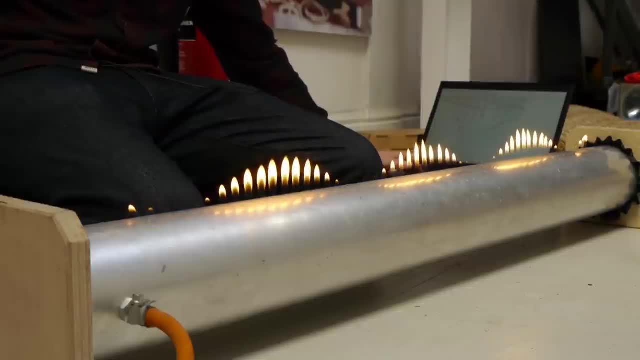 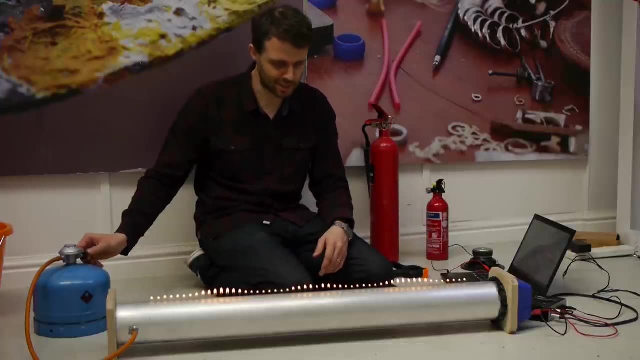 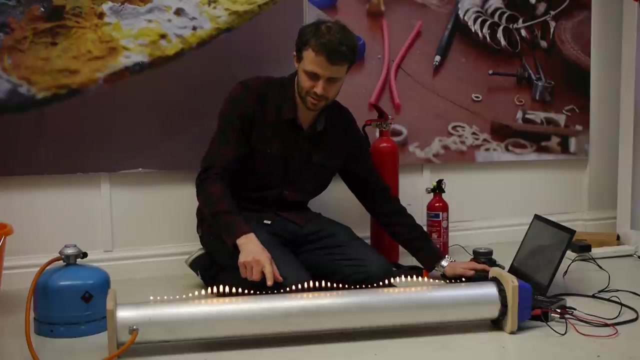 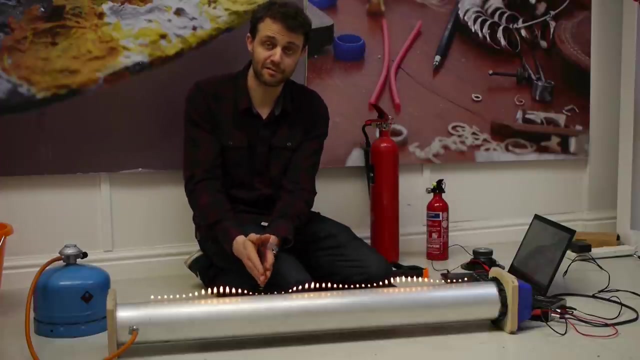 Hopefully you can see the result of the standing wave in the flames. So these points are the nodes. here and here These are the antinodes. So these points, the nodes where the flames are small, those are the points where the pressure isn't varying very much At that point. the tall flames: those are the antinodes. So I've got the pressure. Everybody has those tiny nodes but totally un jakim to hook up with the high flame. Those points are essentially py�도ite pressure. You don't know where those layers are going up and down. 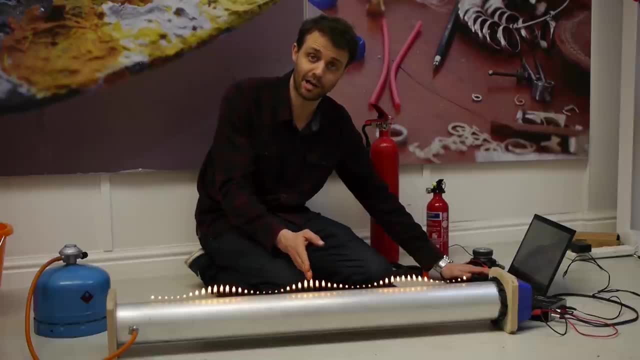 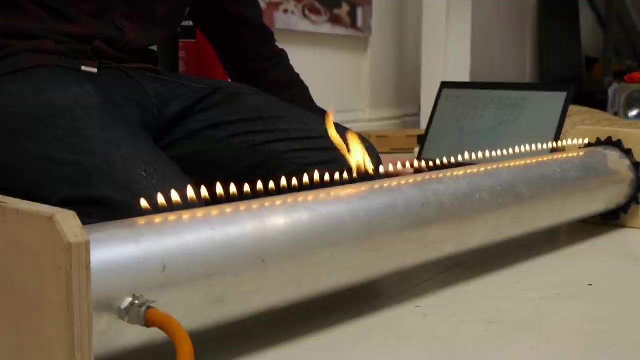 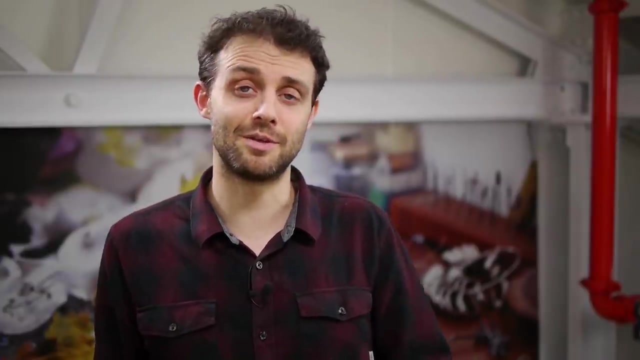 the anti nodes. those are the points where the pressure is varying a lot at that point, and let's see if we can find some higher ones. I swept through a few there. let's see what we've got, and that is the Rubens tube. so what's all this got to do with the sound that? 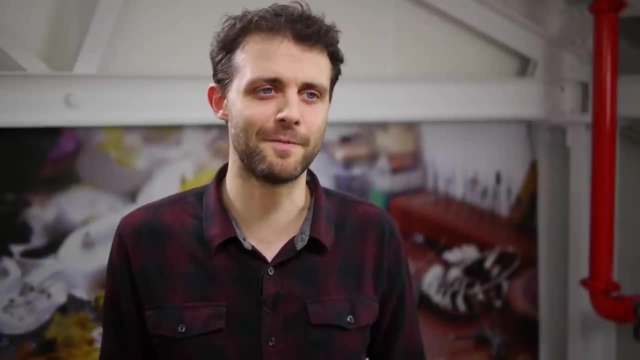 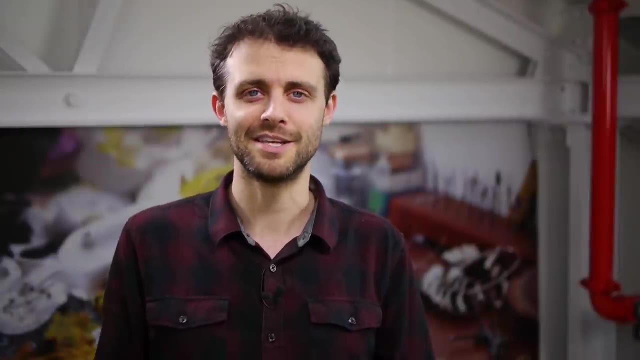 something makes when you're playing with it and you hit it or pluck it or blow over it. well, any scenario like that you come across needs its own explanation. so let's look at one particular example. let's look at wind instruments. so I've got my wind instrument here. it's a 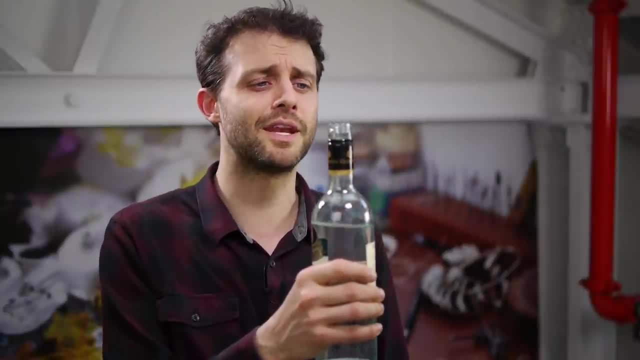 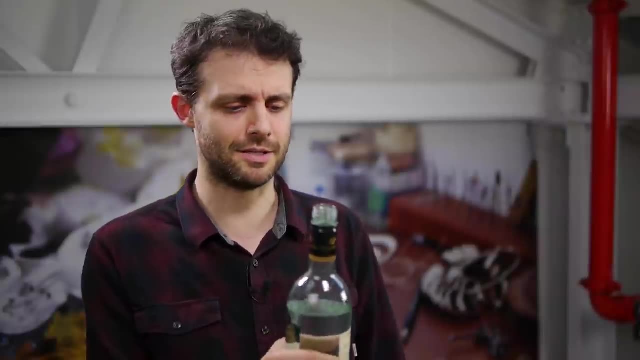 bottle and I've filled it with water and I can blow over the neck like this. when I do that, I get a nice note. so why does that happen and how does it relate to resonance? so when you make that noise with your mouth, that kind of noise- 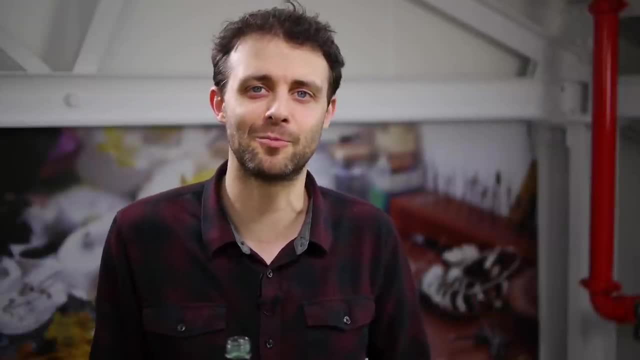 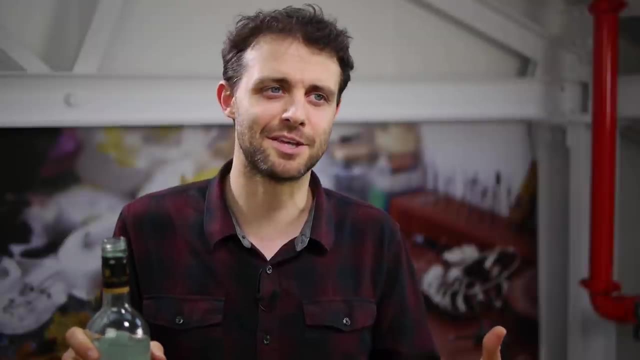 that's white noise and you may have had a lot of trouble with that noise. and you may have heard white noise being described as a mixture of all frequencies within a range at the same time. so when you get that kind of hissing, whooshing sound, it's a whole range of frequencies all jumbled up. 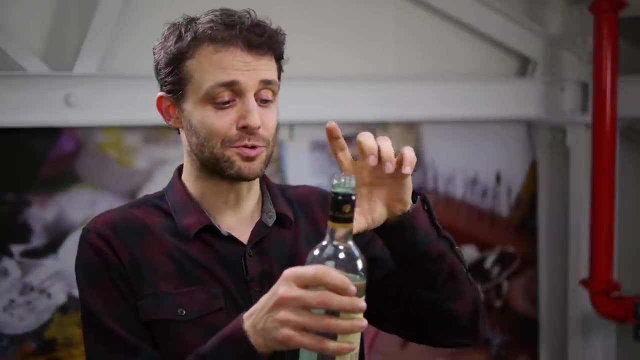 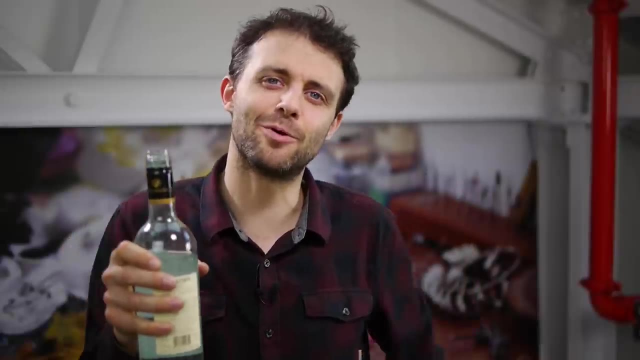 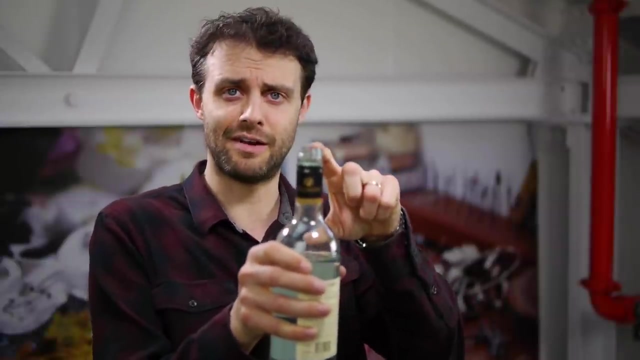 together. so when you blow over the neck of a bottle, you're driving the body of air inside at a whole range of frequencies, but because of what we learned with the Rubens tube, it's actually only the resonant frequencies of the bourbon- the body of air inside- that get amplified. 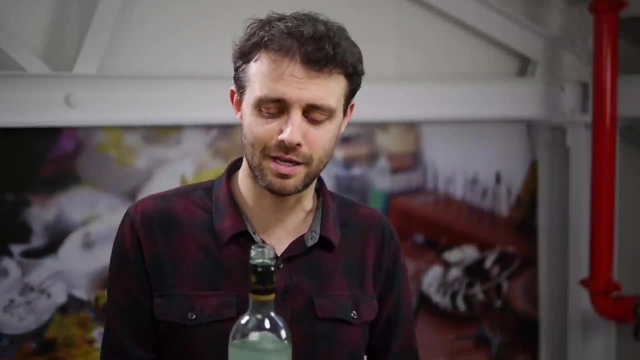 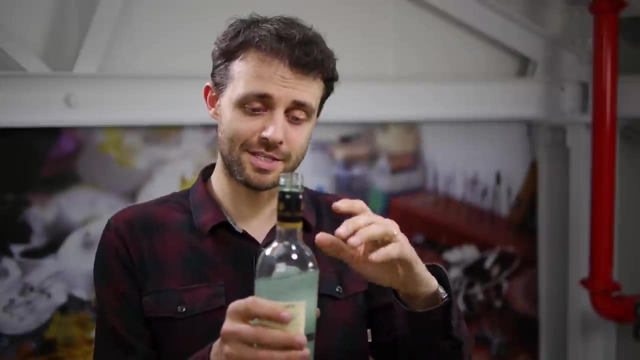 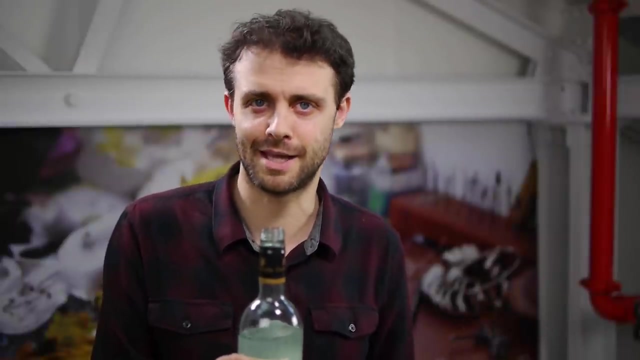 And so those are the ones that you hear. Interestingly, when you hear a wind instrument, you perceive the lowest resonating frequency, And all the other frequencies that are being generated when you blow over the neck of a bottle like this just add to the timber of the sound. 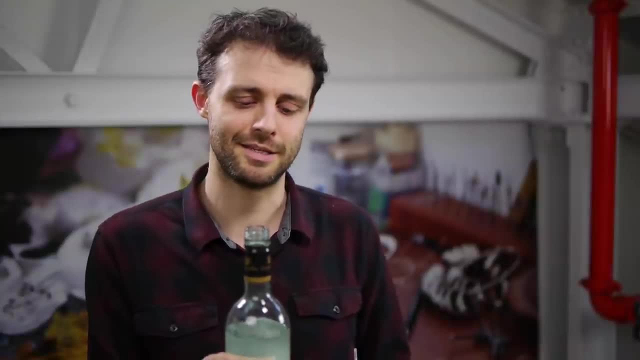 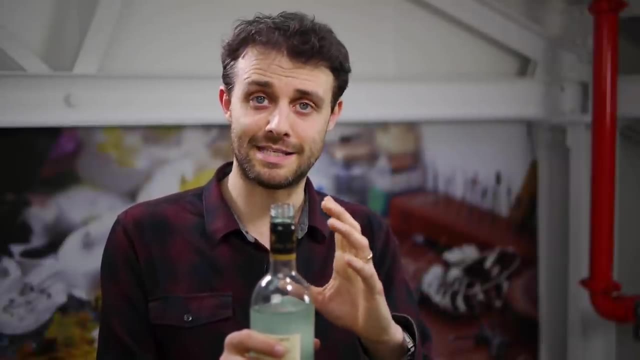 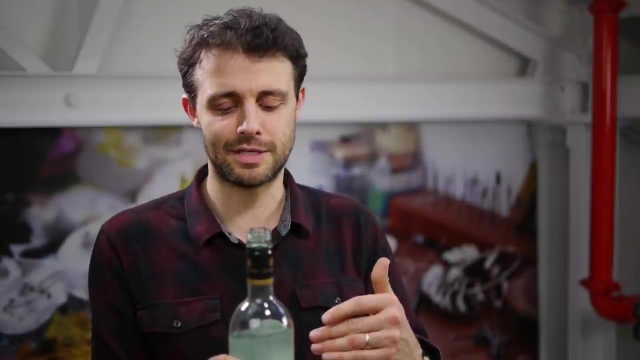 They don't change the perceived pitch of the sound. So the quality changes, the timber changes, depending on the balance of the resonating frequencies that are generated. And it's this balance that helps us to distinguish one instrument from another: The case of a guitar string being plucked. 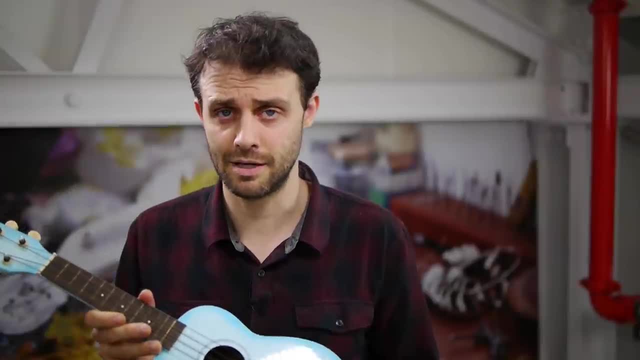 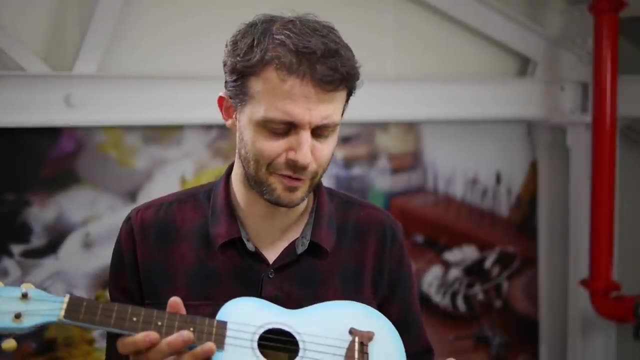 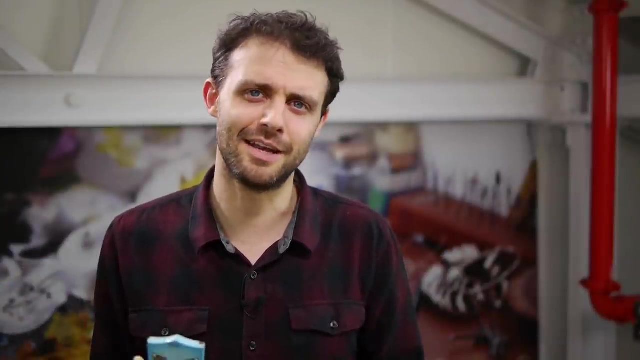 is a bit more. it is a guitar actually, I'm just massive. The case of a guitar string being plucked is a bit more complicated. It involves things like Fourier analysis and stuff like that. It's really interesting and I may cover it in a future video. 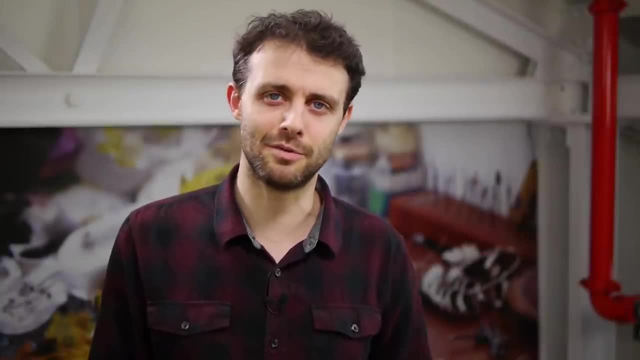 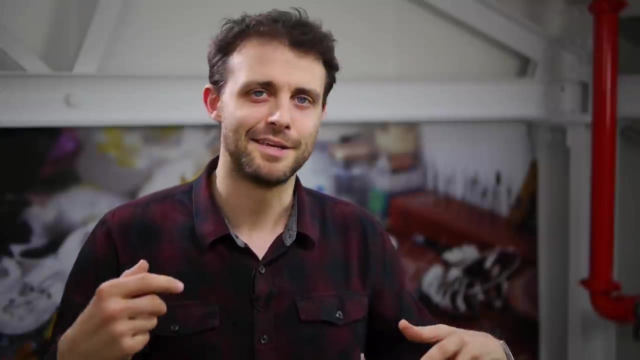 But for now I'm going to leave you with the Rubens tube responding to music. But before that, if you're interested in learning more about wave dynamics and resonance and sound and that sort of stuff, then I can recommend an online course. 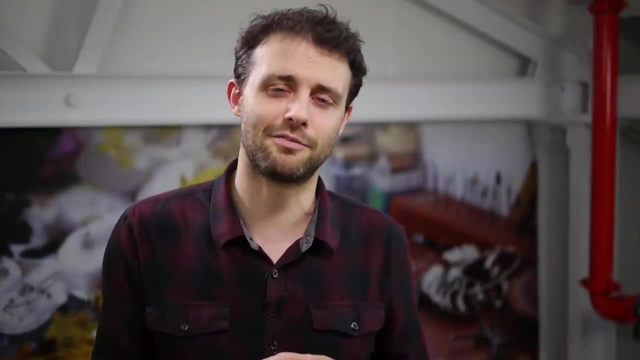 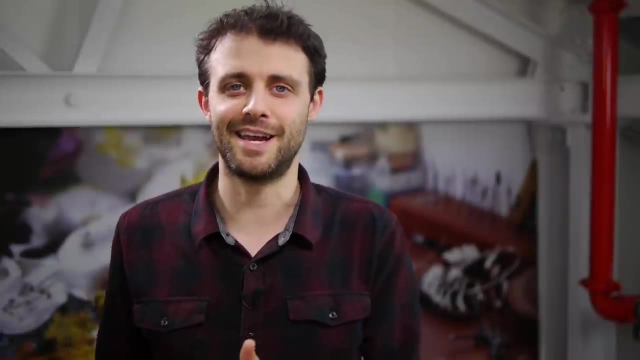 It's called Physics and Our Universe and you can find it over at thegreatcoursespluscom. I'm grateful to The Great Courses Plus for sponsoring this video. If you want to see, for instance, the Great Courses Plus- Physics and Our Universe, the course for free. 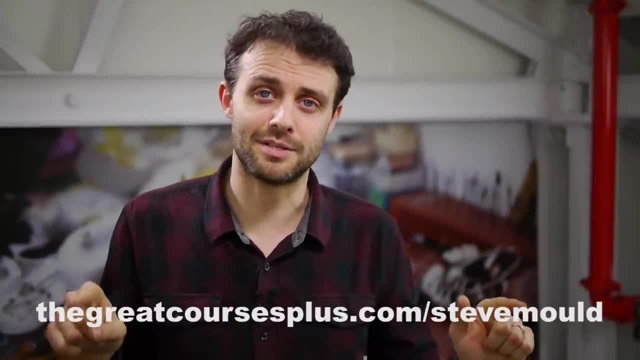 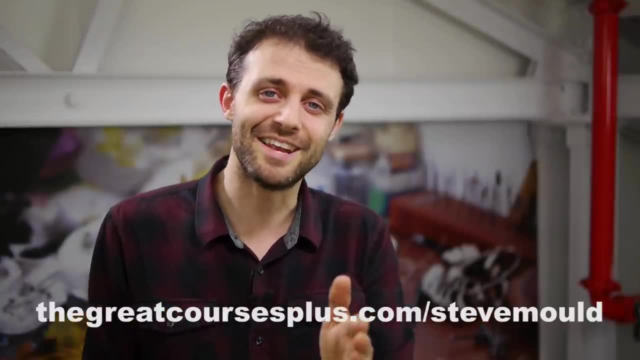 then you can sign up for a free trial at thegreatcoursespluscom. forward slash Steve Mould or click on the link in the description. If you use that URL or the link in the description, then they know that I've sent you. 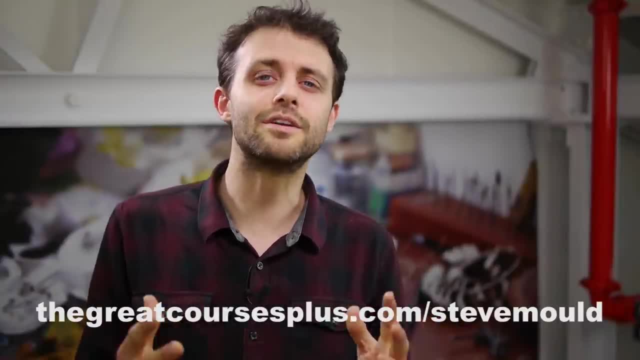 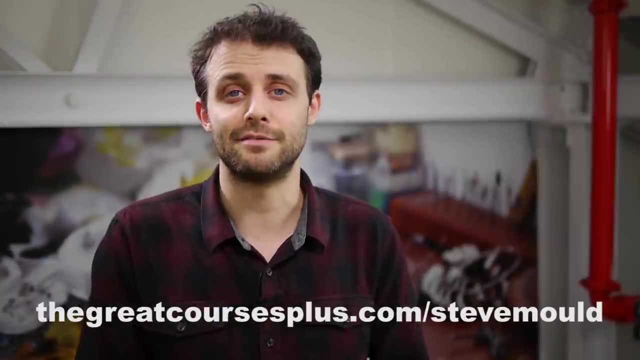 which really helps me out. The Great Courses Plus is an online on-demand video learning service, And if you sign up now, then you'll have unlimited access to 7,000 plus videos from top-notch lecturers and experts on the subjects that you love. 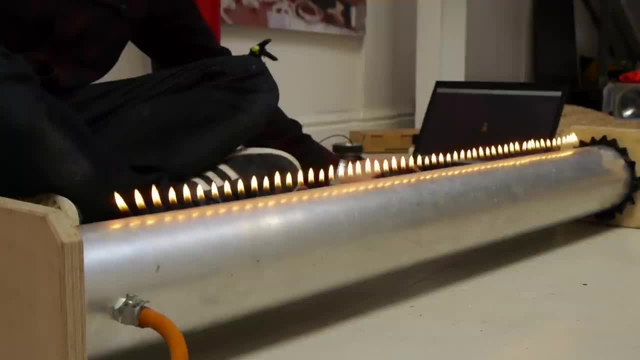 In your case, probably science and maths. Not just mathematics, not just magic. It's all about the universe. This course is meet-and-de-sense training and I hope you have a great time. I hope you enjoy it And don't forget. 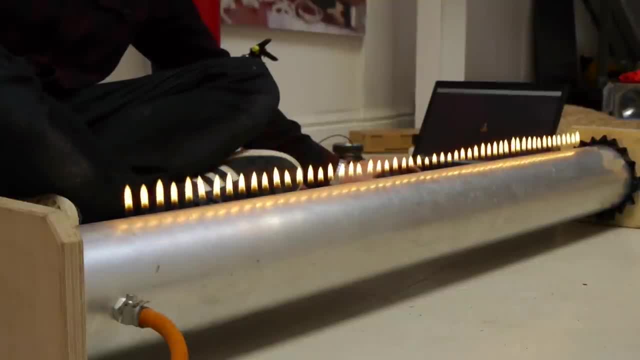